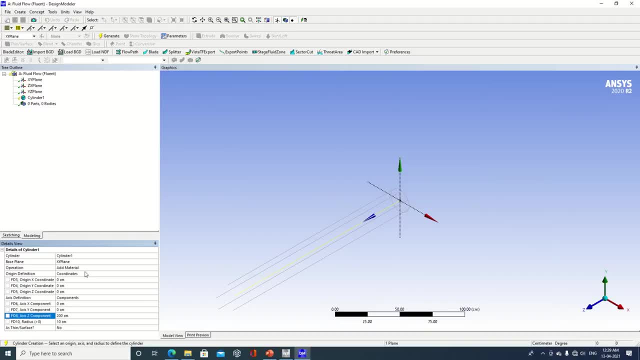 in z So you can see the wireframe model over here. So this is, I will make it generate Now. in this case, you are not able to see this object as a transparent one, So I will go for the option which is called as frozen, So now you can see inside of your object also. 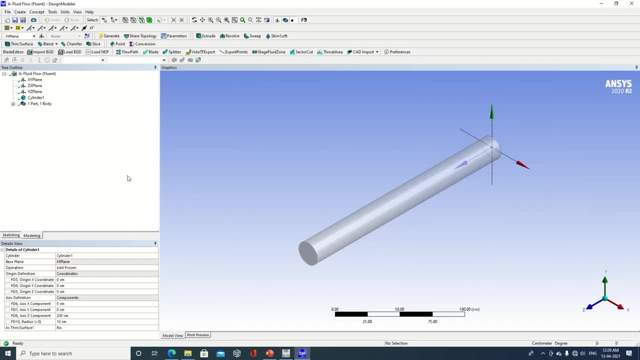 One more thing. what is important? here? you can see one part, one body. Now we want a fluid which is flowing through the pipe. That's why you want to create this pipe with a hollow. So I am going for this as a thin surface. So I will make it S and make it generate. 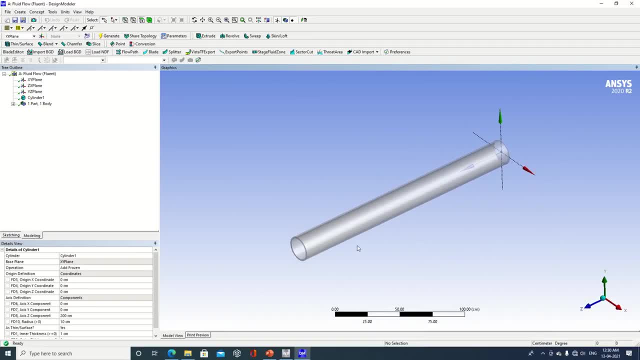 Now this has been created as a whole object. Now the computer is running out of the lags, doesn't understand which one is. where is the fluid is flowing, where the wall will be there. so accordingly, if you have to specify the fluid and inside. so now I. 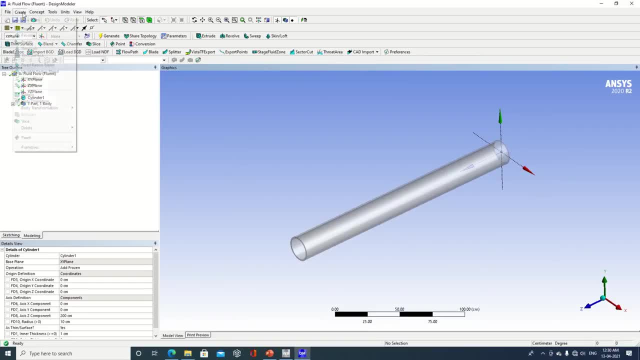 will. what I will do here over here is go for the field operation over here. so I will select this internal part, make it apply and I will generate now. earlier it was one part, one bodies. now it is two parts, two bodies. so second one- I will specify this as a fluid because we want to do analysis on fluid. so first one. 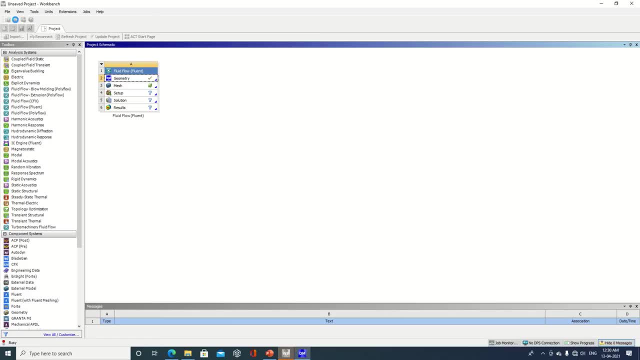 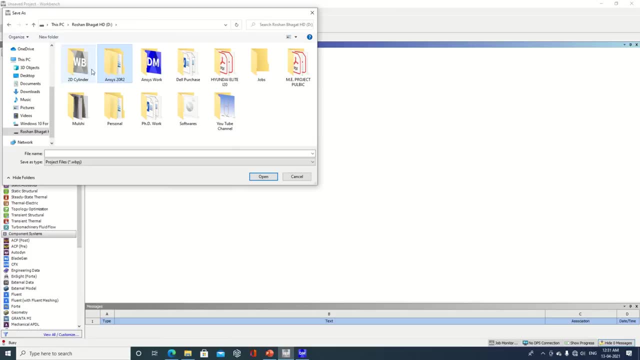 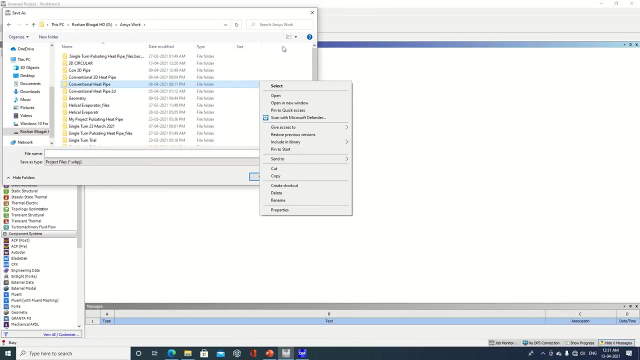 this is solid wall and second one it is a fluid. so this is has been completed, so I just go on to save this work over here. okay, we should save with the different name to: ok, so this has been saved. now you can open the next part, which is related to: 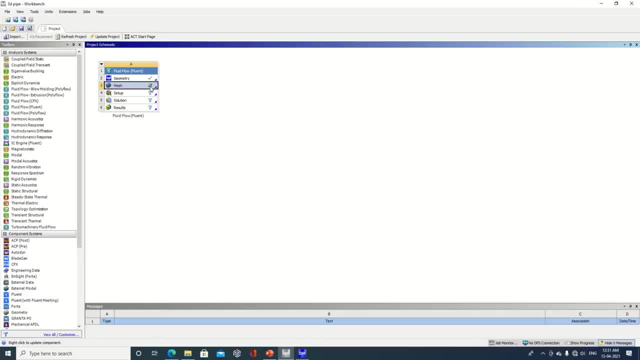 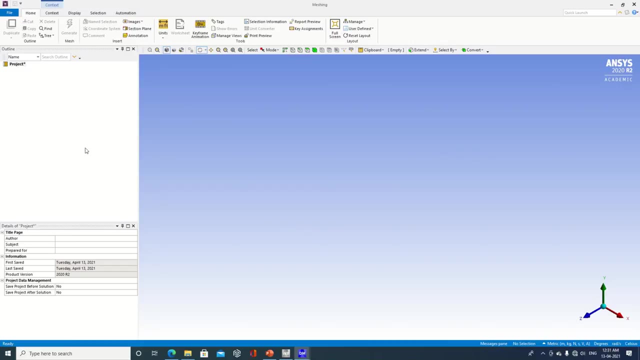 the superide吗? ok, so this has been saved. now you can open the next part, which is related to on the mat. it is the heute, it is the everyday, it is behalf. it is alsodies related to mesh here, to select either fine mesh or to select. we say, you can have coarse mesh. 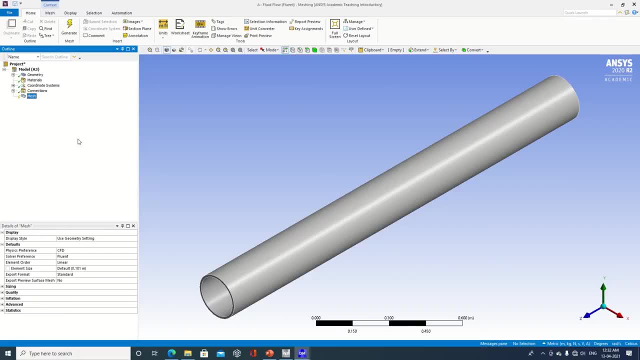 also so, depending on we say how much size you are taking now, at the present, you will also. this is 0.1, so you can just go to the static stick once the mesh is being generated. so say, I just make it update so you will see some mesh. 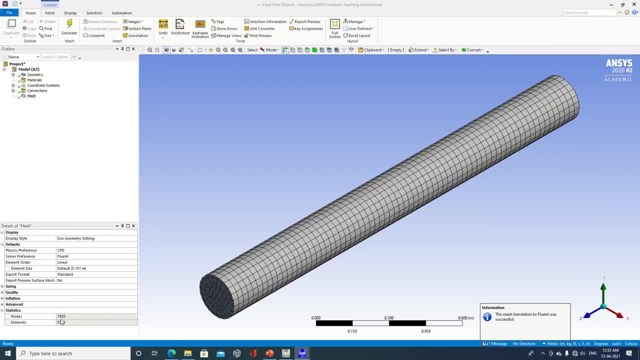 has been generated, so 7920, quite low value as far as the academic version is concerned. you can use it for file act. well, thousand it. we can say number of node points. so I can increase this value to some higher value: 0.01. so we'll make. 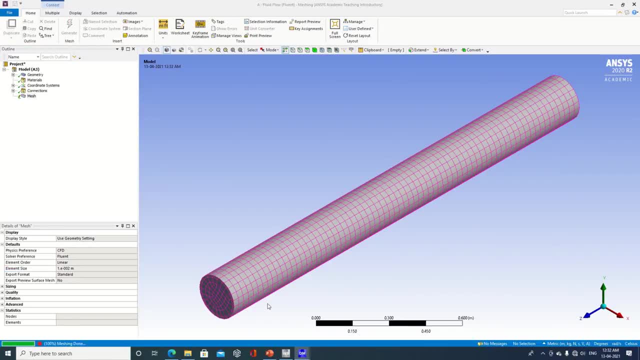 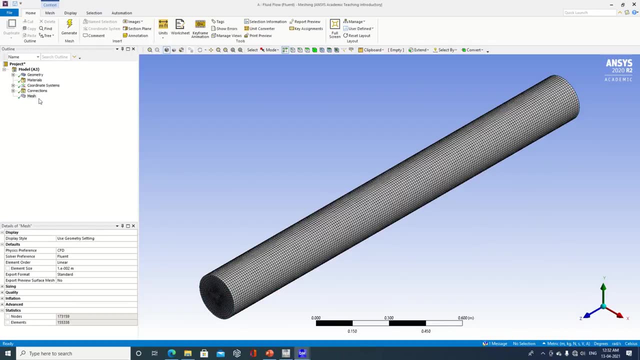 it again, update so that the mesh will be generated over here. so I'm taking the size so that it will not take much time, as as computational time we want to reduce, so accordingly. now next thing will process will be to specify names. so here the computer doesn't understand which one is inlet and which one is outlet. so 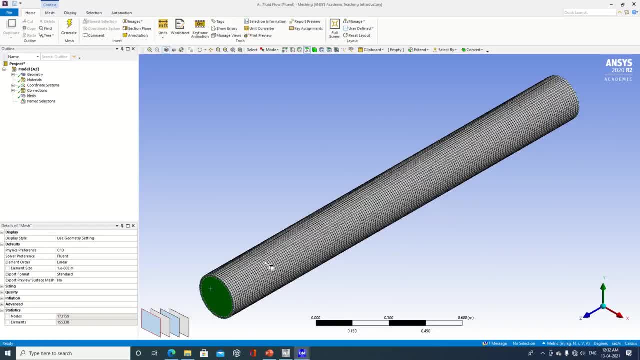 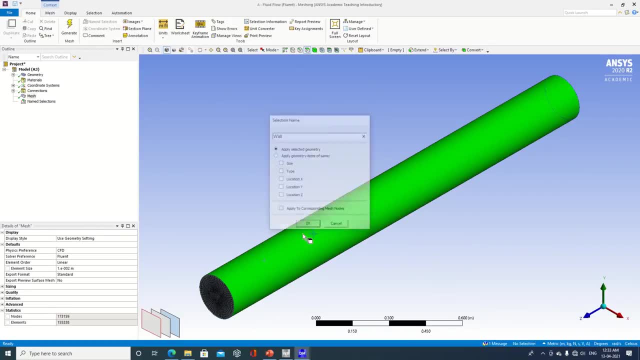 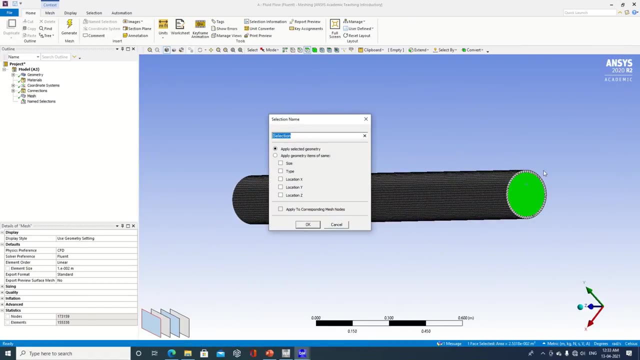 we have to specify inlet and outlet over there. so this will be my wall, so I am selecting this as a wall and the other end I will specify this as an outlet. so first one, I have specified inlet, then I have specified wall. now I will specify as a. 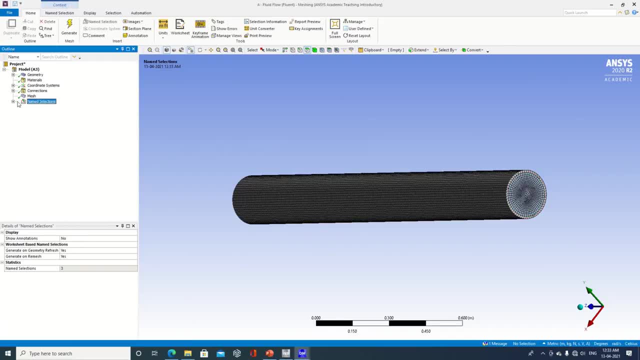 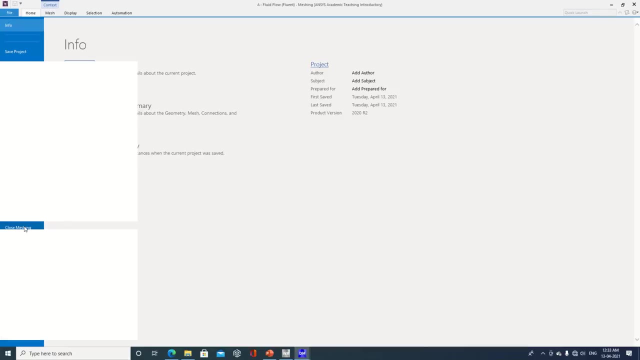 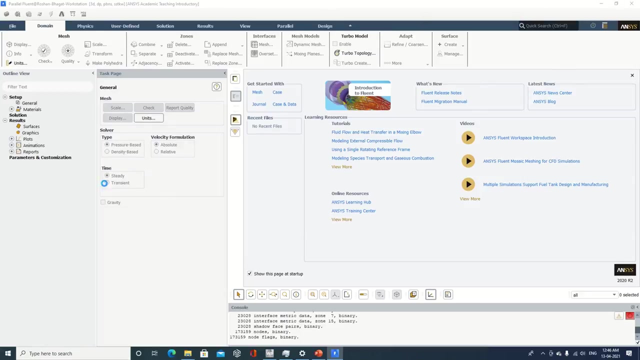 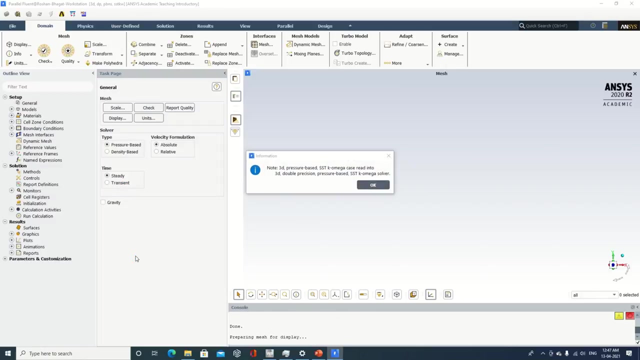 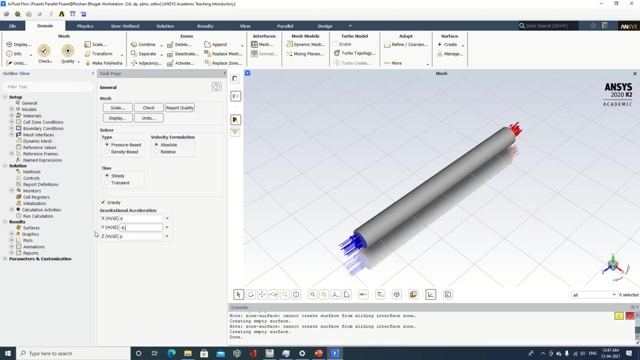 outlet so you can check out here also: inlet, outlet and wall. now one more time. I will make it update so that will message will appear. the mesh translation to fluent was successful. now you can close the here and you can proceed. for the next part, you I will specify gravity: that is minus nine point eight one, and this is a horizontal. 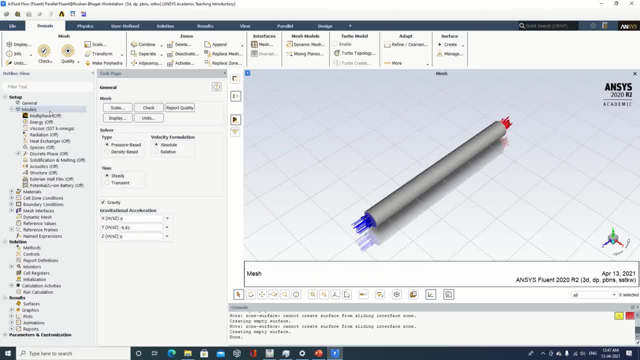 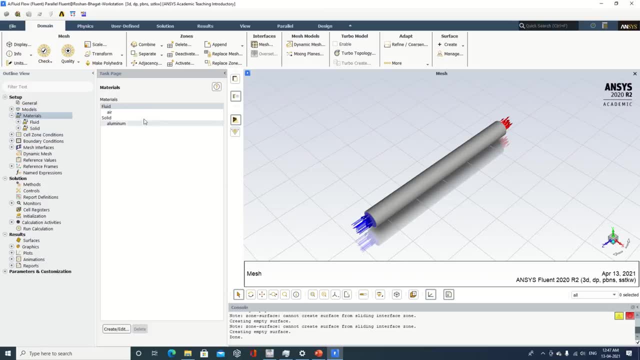 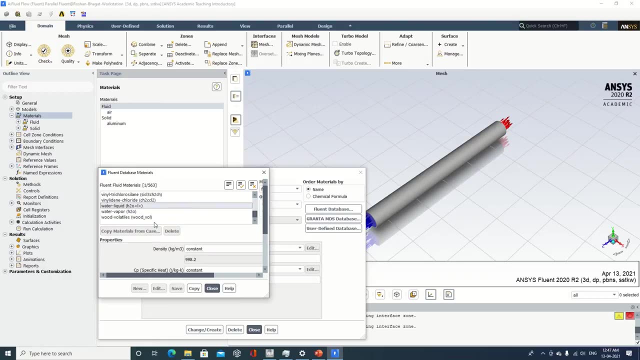 pipe doesn't bother much about gravity, then model: I will keep as it is. nothing I will change with this one, I will just go with the material. in that material I will select water over here from the fluent database. here you can select water liquid. so make it copy, make it close. so close this one. I am not changing the. 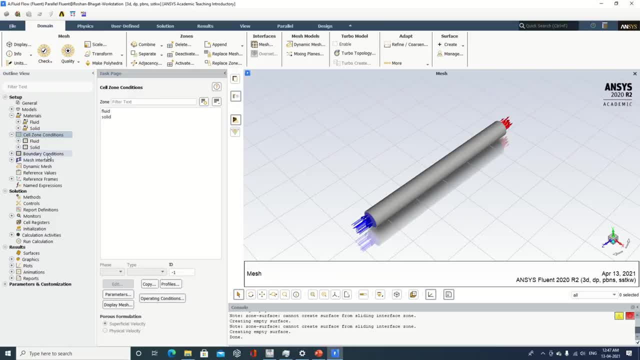 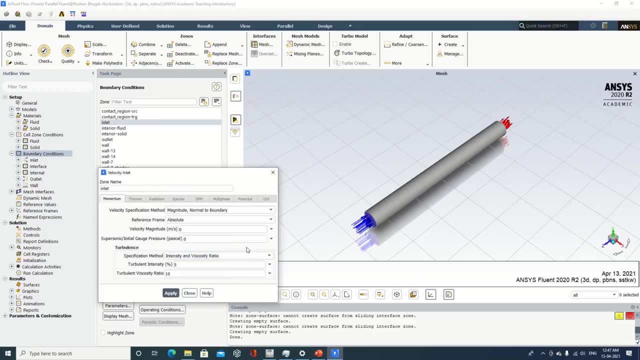 solid also. then cell zone condition: no such changes in boundary condition. I will specify at inlet some velocity say. for example, I will specify 2 meter per second. this is a velocity, then make it apply this one. I will close then going to reference values, I will tell computer from where it's to start. it will compute. 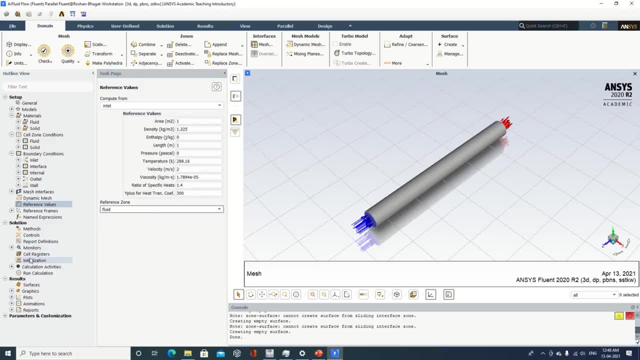 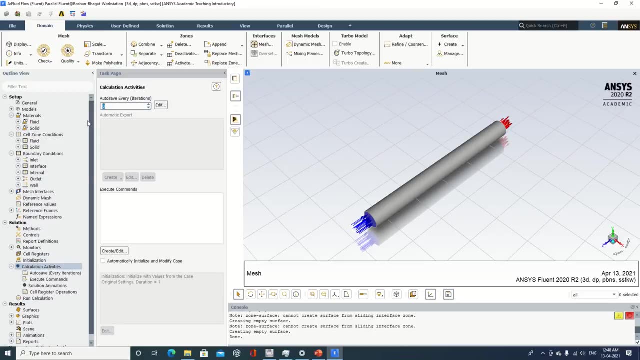 from inlet in the fluid zone. next thing will go for the initialization. we say we will go for standard initialization. I will tell again computer from where it should start. I will say inlet. then going for the calculation activities, I will specify the saving point over there. then solution animation also you can set at. 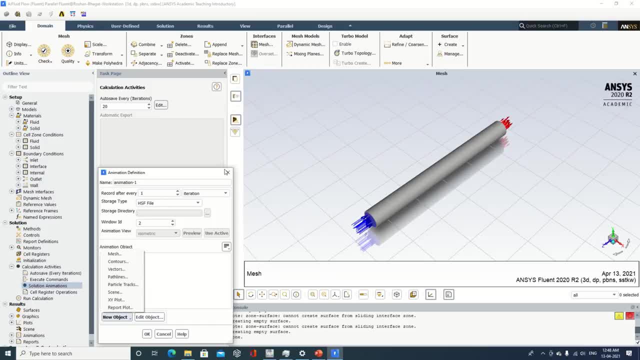 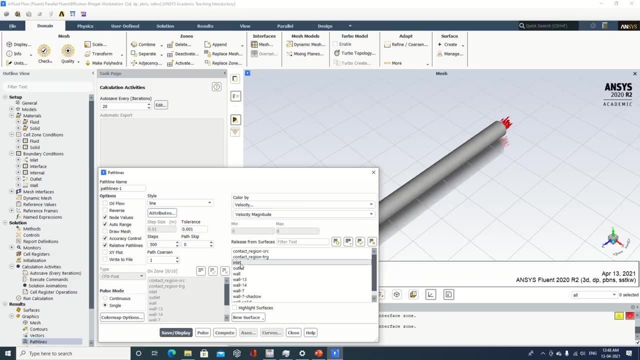 what we can say if you want to save the animation. so this also one thing which can be done, otherwise you can skip also. so here go for the graphics. in that graphics select path line. now which variable we are interested in: velocity, velocity magnitude at inlet, outlet and wall. so specify that, then you can just check it. 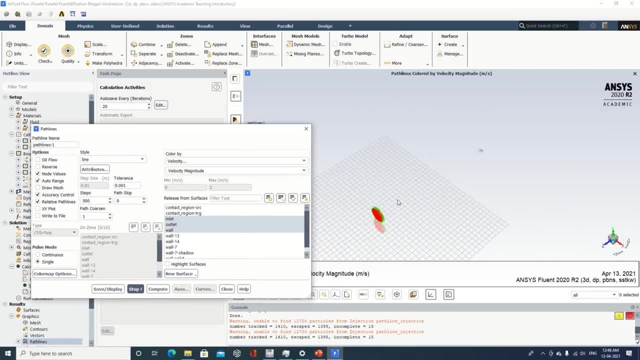 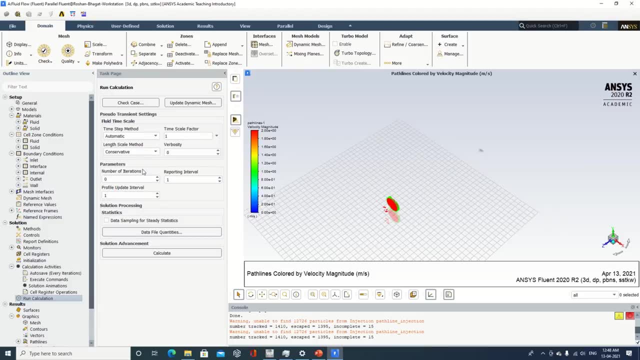 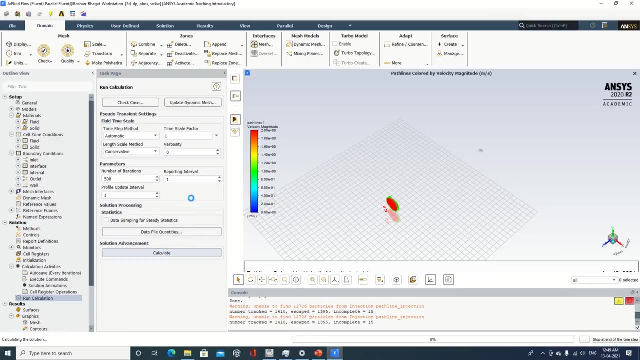 out the pulse also. so here, if this is going forward, it means whatever you are done is correct. you can stop it. so this is part which has been done. going for the calculation now see, let's enter the number of iterations. say, for example, it is 500. now start process. 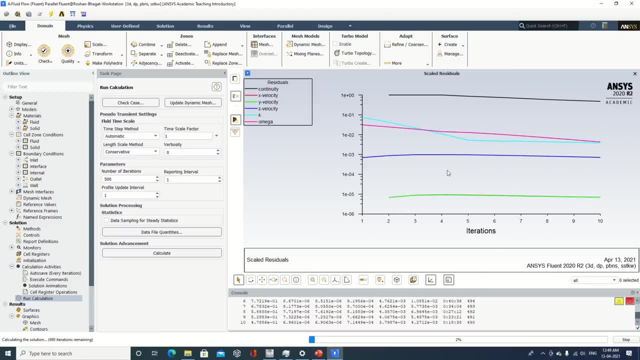 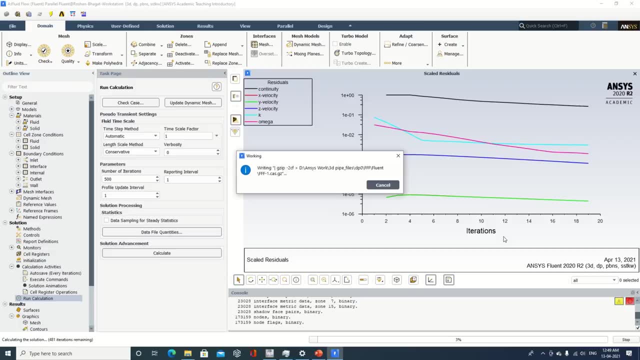 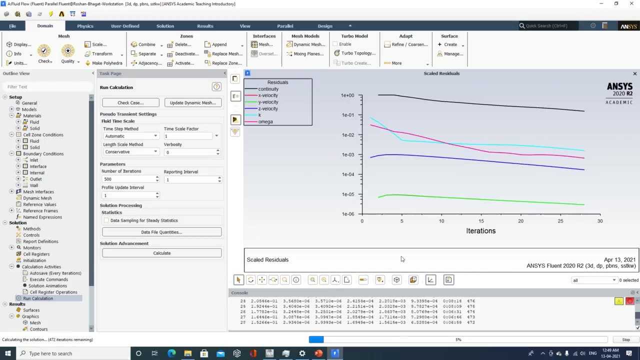 so this has been started at, depending on system, till expiration at will taking time and calculation is completed. the final calculation should be fished in remember below. if you not gain enough, the code clock. further processes can be done. so the message will appear here as calculation is completed. so, depending on system configuration, also depends on that. the 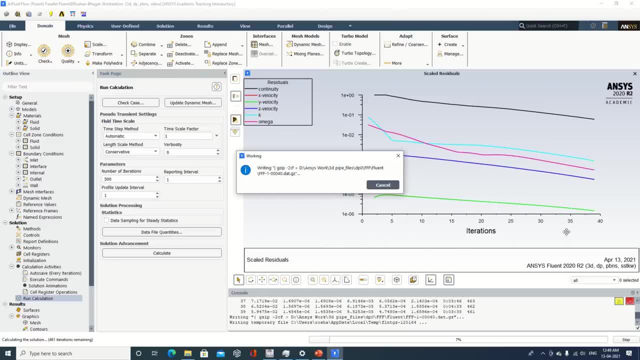 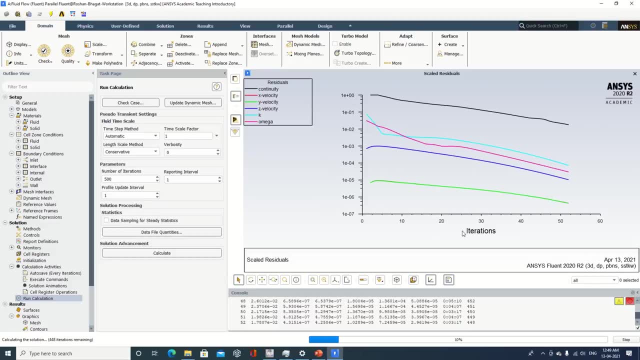 size of mesh you are selected. the time required will be a different for the different system. now this is. you are observing the iterations on x-axis over here, so the console window will show you the number of iterations which has been there. additionally, you can set animation also means the fluid flow. 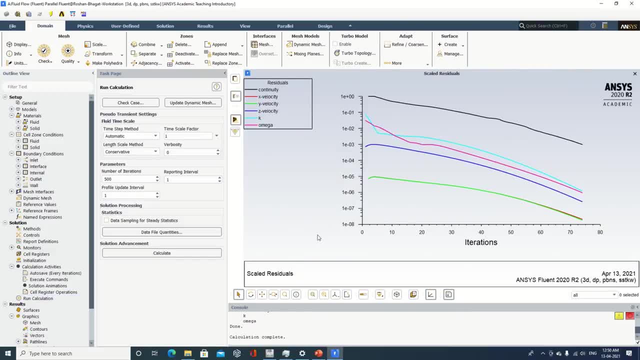 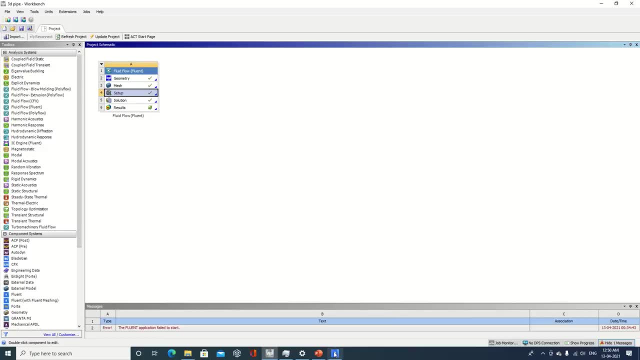 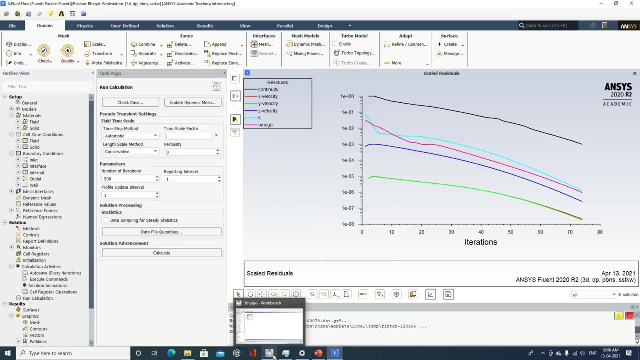 behavior. you can also check it out now here. the calculation has been completed, so now you can just go back to so setup and solution. if it is a right click, you can close the fluent window. so now I can close the fluent window. once the fluent window is closed, you can go back to work. 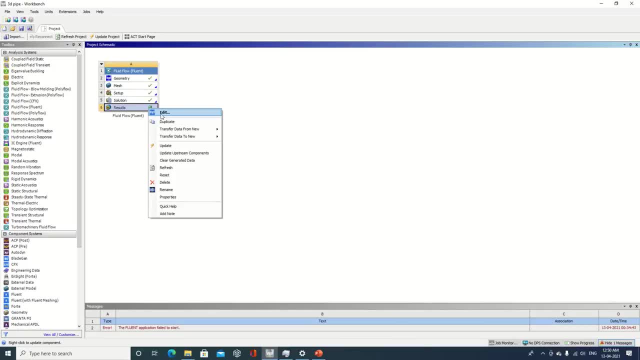 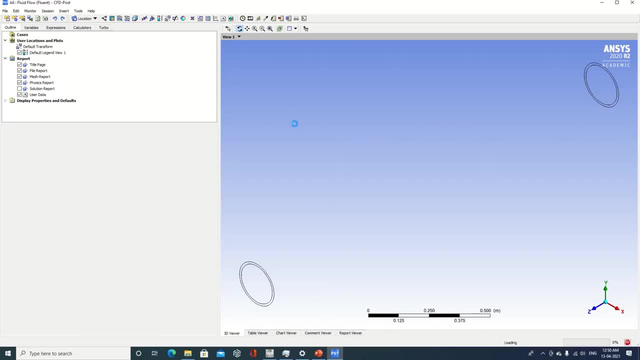 bench window again, and you can go for the last one. that is the result. now, what is in result? in result, you will be able to plot the charts, as well as you will be able to see the conditions at the inlet outlet. now what we have to do is: 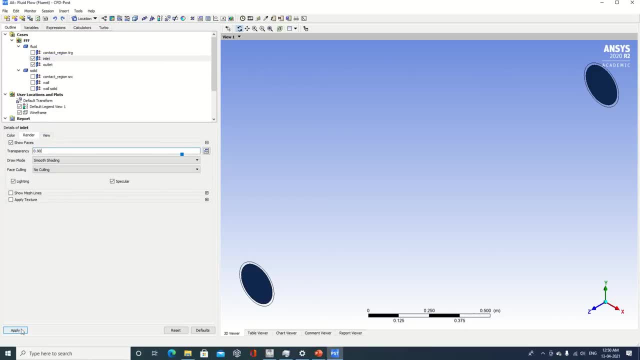 we will set some transparency over here so as to visualize the object properly at outlet also. I will specify the transparency over here: that is 0.9. another thing: this is a wall, so this will allow you to see the transparency of the object. so this will allow you to see the. 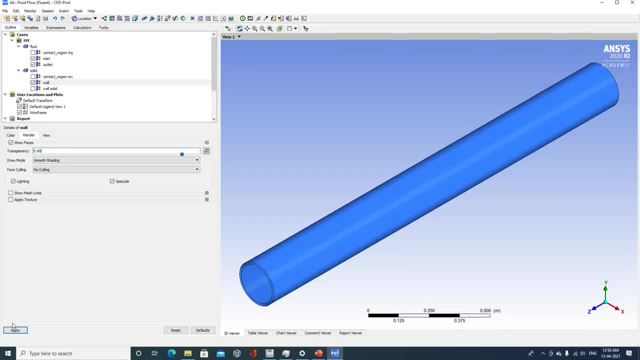 also, I will specify transparency. at this point that is equal to 0.9, and last one, a wall solid. so here also I am going to set the transparency 0.9. so now the object is clearly visible. if you want to remove this wireframe, that can also be. 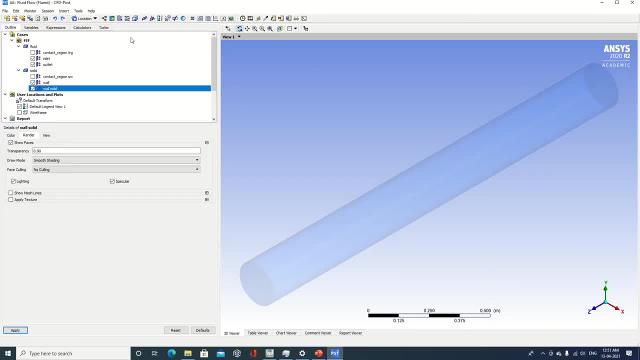 easily removed. now next thing will be to analyze the things which we are interested in. so we are interested in a stream line, so I am selecting a stream line over here. so here I will select it from inlet, so it will start from inlet and it will go towards the outlet. now there are 25. 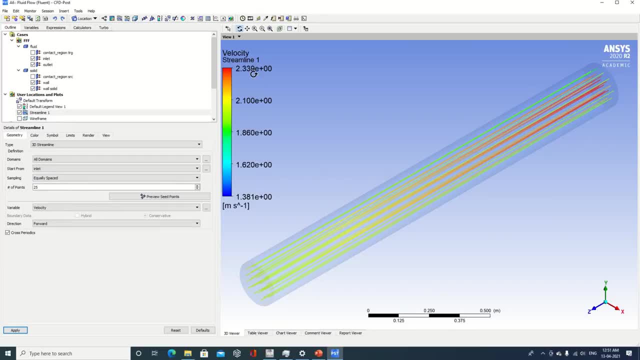 points which are selected accordingly. this will be there. so this is a stream line which is on this side and you can see this is a pipe over there. now, additionally, few more thing we will do. I will give some names over here, so I will specify, let's say, the file name. so specify fluid flow simulation. 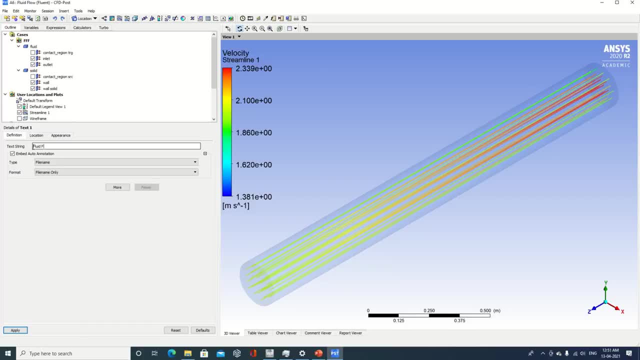 in 3d circular pipe fluid flow. okay, I specified fluid flow simulation in 3d circular pipe, so where I want I want this to be, let's say, for example, central top, I will specify this one. now, the legend. whatever we have, we can either reduce the size of this legend.